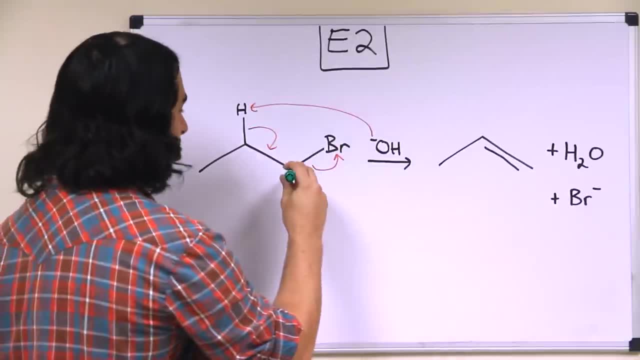 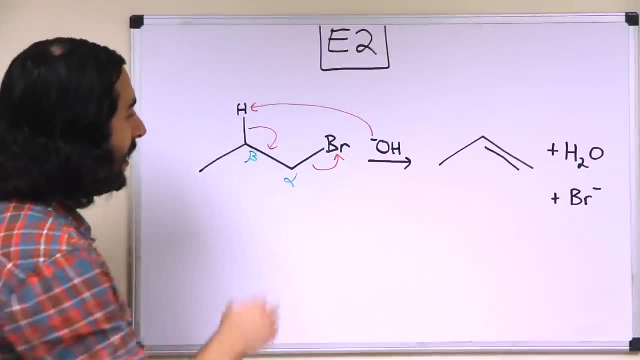 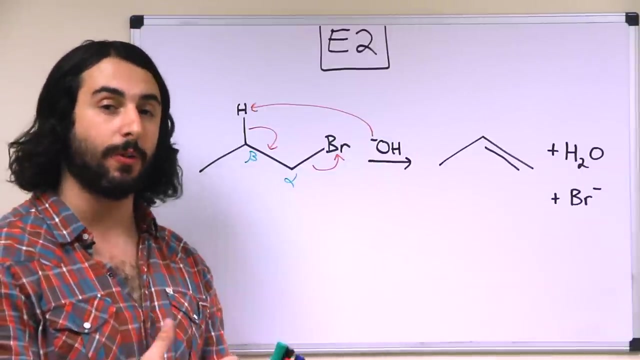 meaning, if this is the leaving group here, this is the alpha position, this is the beta position. it is a proton on the beta carbon that is removed, because it is not going to work out to remove a proton at the alpha position, because then those electrons will have nowhere to go. 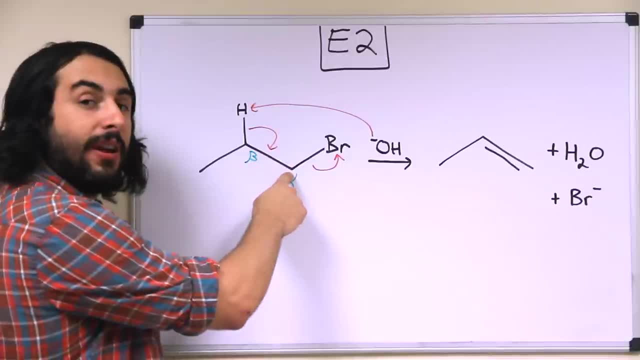 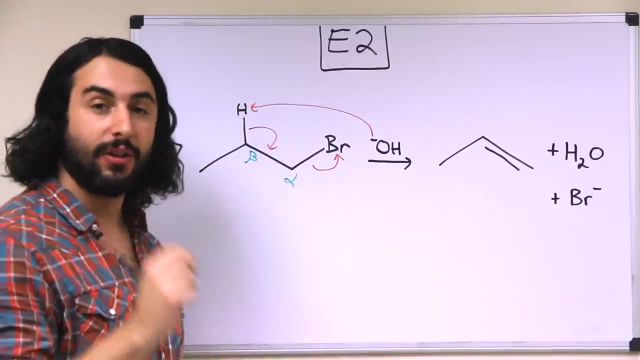 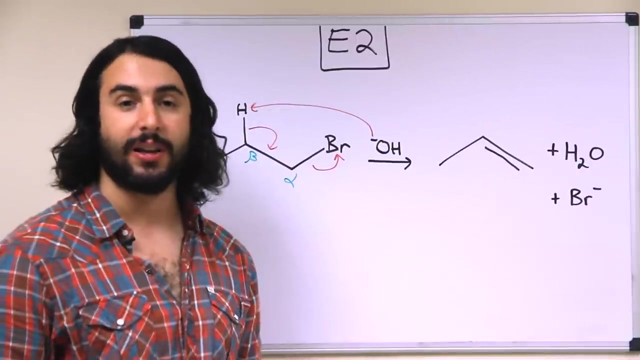 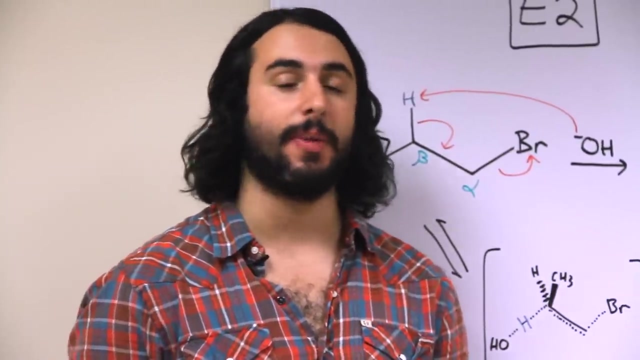 Instead, what happens is that this carbon is able to receive the electrons in this carbon-hydrogen bond, which are the electrons that form the pi bond, because this carbon can also lose the electrons that are now belonging to the bromine. So let's take a look at the transition state of this reaction to better understand the mechanism. 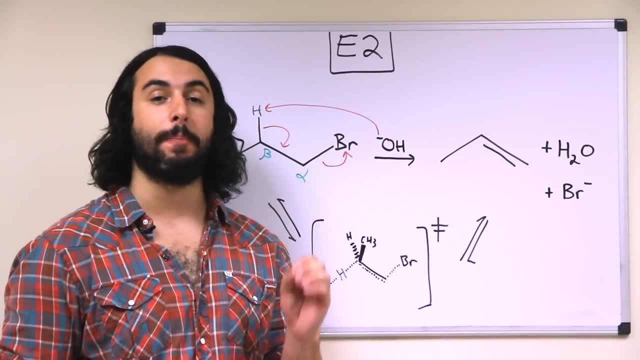 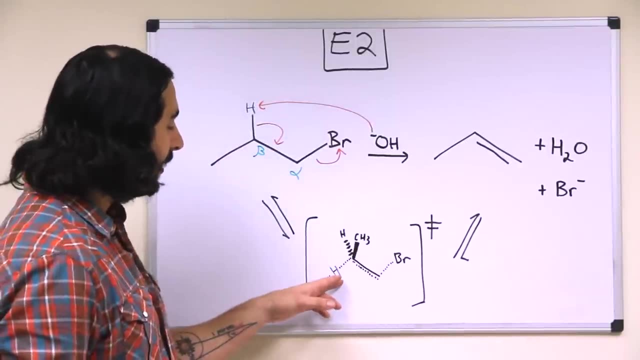 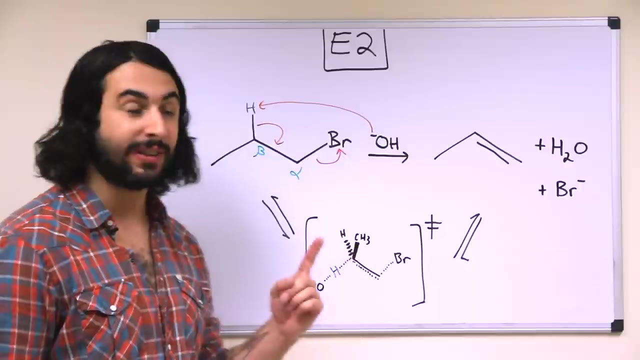 So, just like the SN2 reaction, the 2 is referring to a bimolecular transition state, meaning that the substrate is attached to both the leaving group and the proton that's being extracted at the same time, making this a concerted reaction. It happens all at once, in one step. 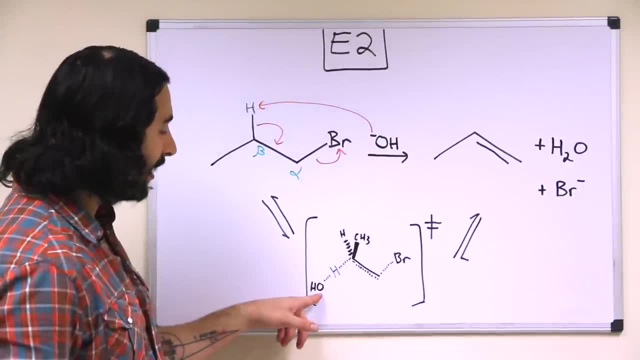 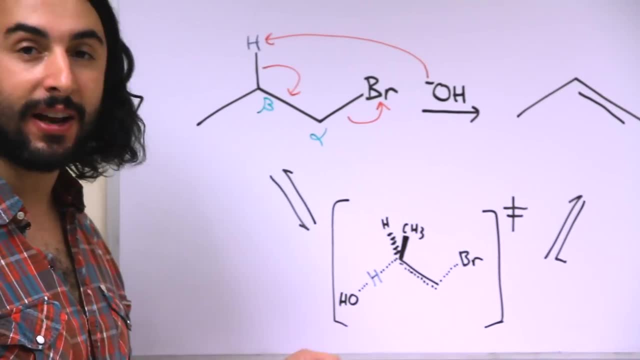 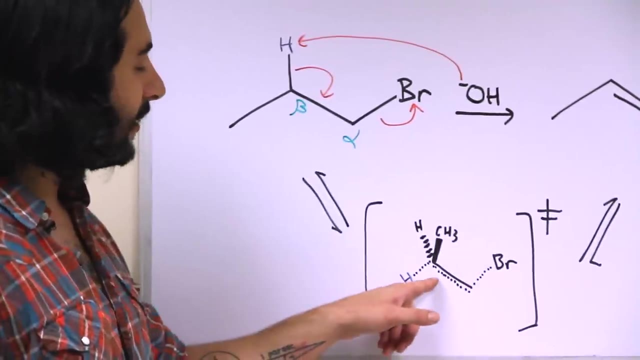 So here we can see that the hydroxide is weakly forming a bond. This is the bond to the proton that's being extracted. as the bond between the proton and the carbon is weakening As well, the bond between the carbon and the leaving group is weakening and the pi bond begins to materialize. 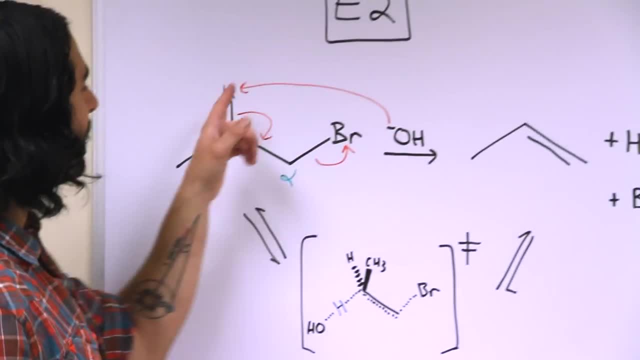 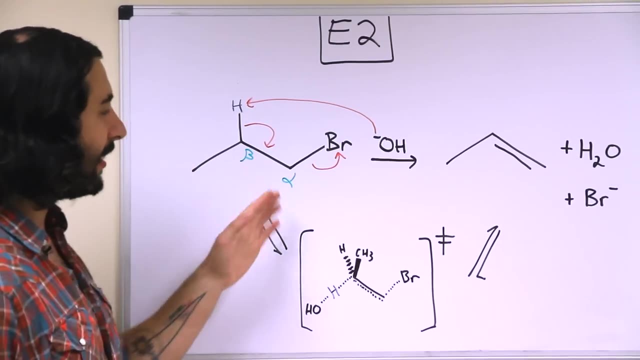 So this happens all at once. It is not the case that the hydroxide extracts the proton, then at a later time the electrons go to form the pi bond and then, once the pi bond is being formed, the carbon realizes it has too many bonds and loses the bond to the leaving group. 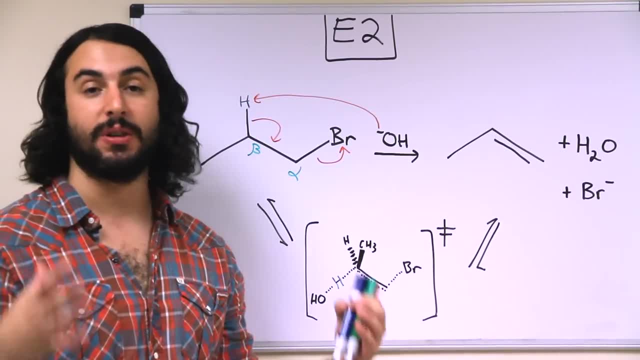 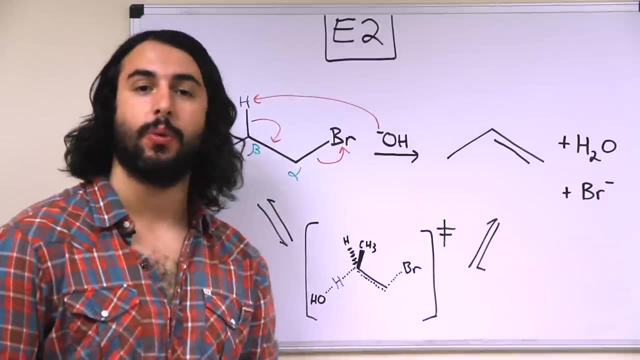 That's not the case. In fact, all of these bonds are materializing and dematerializing at once, So there's the transition state and then the final product with the pi bond in place. Thanks for watching, guys. Subscribe to my channel for more tutorials. 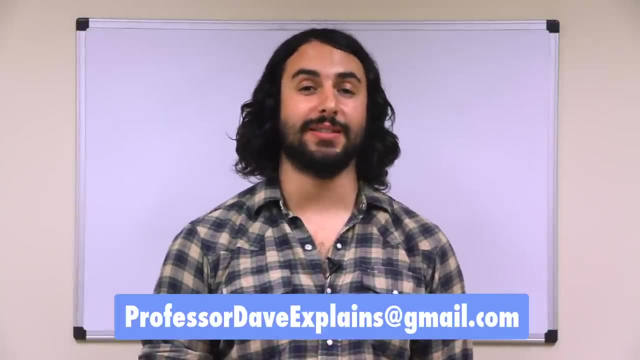 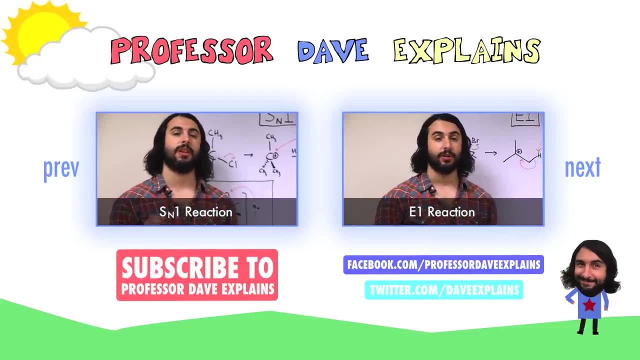 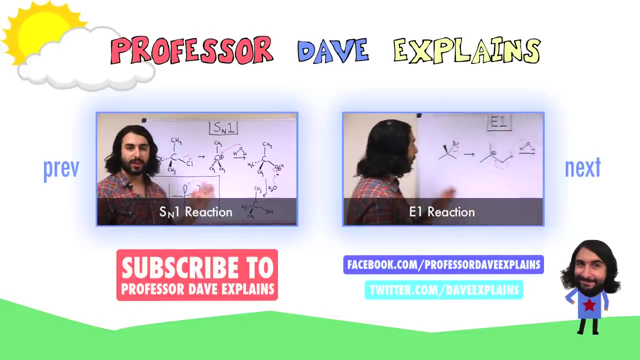 and, as always, feel free to email me with questions professordaveexplains at gmailcom. I'll see you next time.